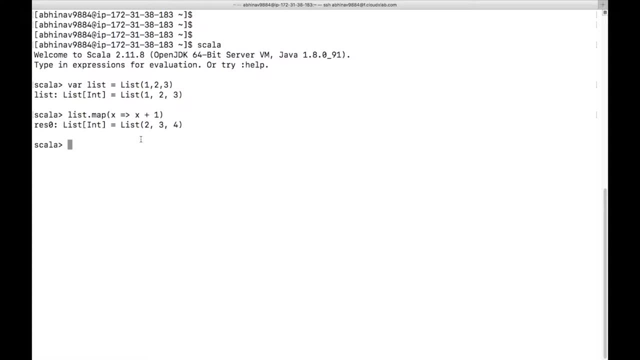 Here map function added one to every value in the list. For every value x in the list, x plus one is calculated. There is another syntax to define map Where, instead of giving a name to every value being used in the function, we use a placeholder underscore to represent the value. 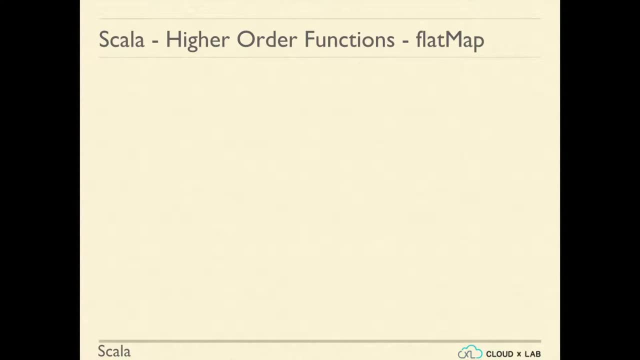 Let's learn the higher order function, flat map. Flat map takes a function as argument and this function must return. a collection Collection could be empty. A flat map is called on a collection itself. The flat map applies the function passed to it as argument on each value in the collection, just like map. 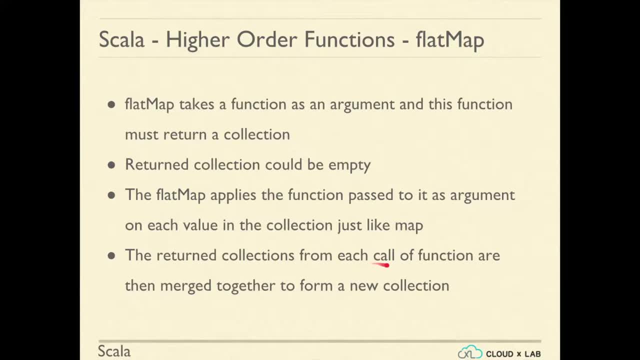 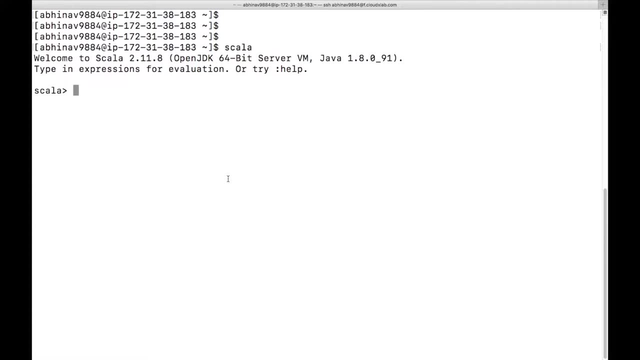 The returned collections from each call of a function are then merged together to form a new collection. Let us understand it with an example. Let's define a list of languages. Type var list equals list python comma- go. Here we have a list of strings. 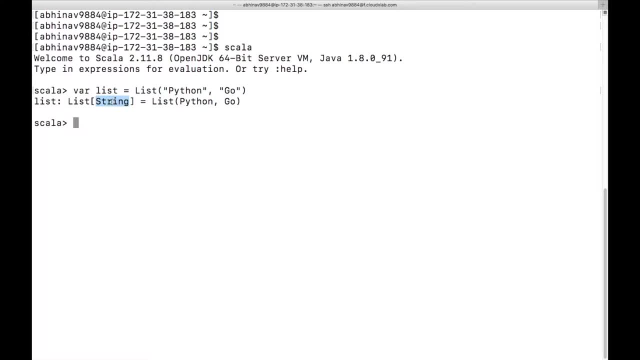 A string is nothing but a sequence of characters. Define a flat map Type list: dot. flat map bracket. lang equals greater than lang plus double quotes. hash Flat map appends hash to every string in the list and then flattens it down to the string of characters. 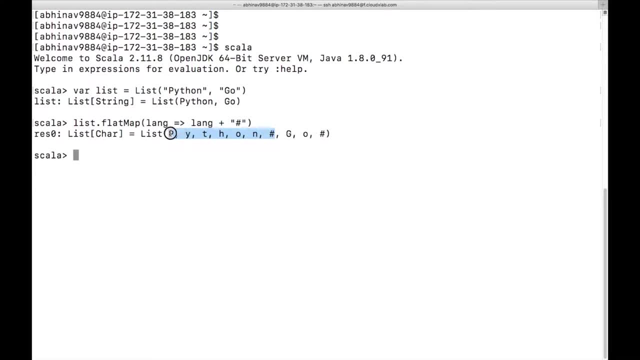 As you can see on the screen, hash is appended to python and go, And then python, hash and go. hash have been broken down into sequence of characters. We can also define the same function using the following syntax: flat map: bracket underscore plus hash bracket, where the underscore is a placeholder for each value in the list. 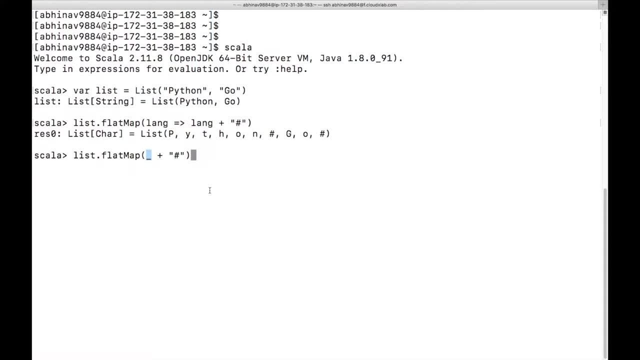 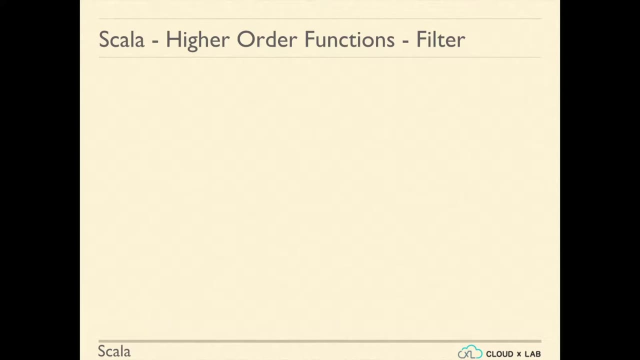 So, as we can see, that the size of output collection could be larger than the size of a collection, While in case of map, the input and output collections were of the same size. Let's learn the higher order function filter. Filter applies a function to each value in the collection and returns a new collection with the values that satisfy a condition specified in the function. 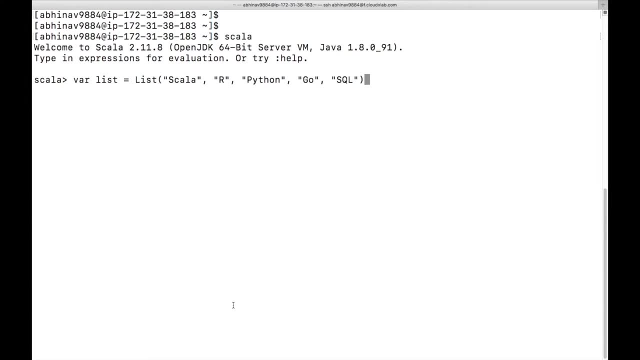 Let's understand it with an example. Say, we have a list of languages- scala, r, python, go and sql- To filter out languages which contain capital S. type list dot filter: lang equals greater than lang dot contains s. As you can see, we have a new list now with only scala and sql as the values. 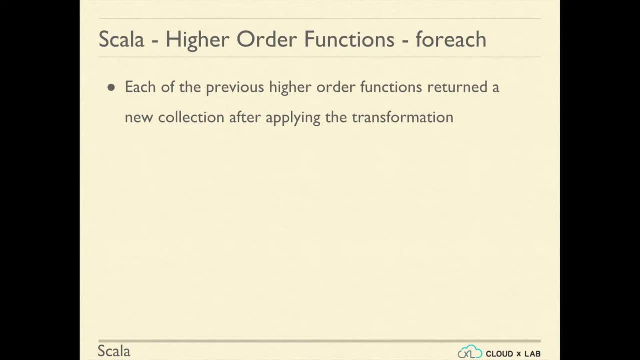 Each of the previous higher order functions returned a new collection after applying the transformation or filter, But at times we do not want the functions to return a new collection. It is a waste of memory resources on JVM if we do not want a return value. 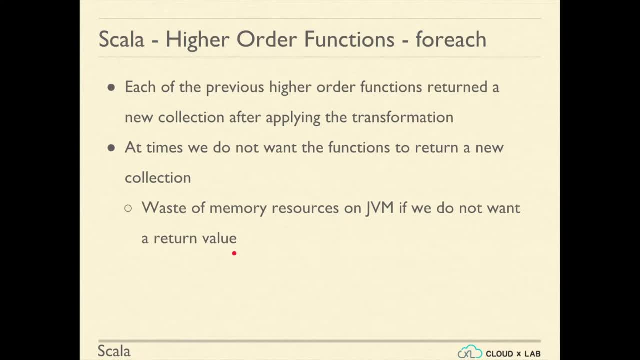 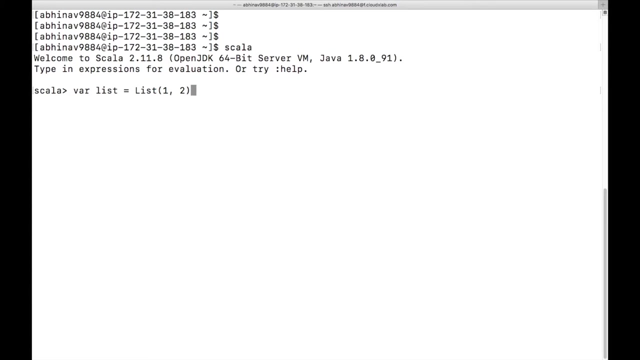 Higher order function, such as foreach, allows us to apply a function to each value in the collection. But we can also apply a function to each value of a collection without returning a new collection. Let us say we have a list of values 1 and 2 and we just want to print each value in the list. 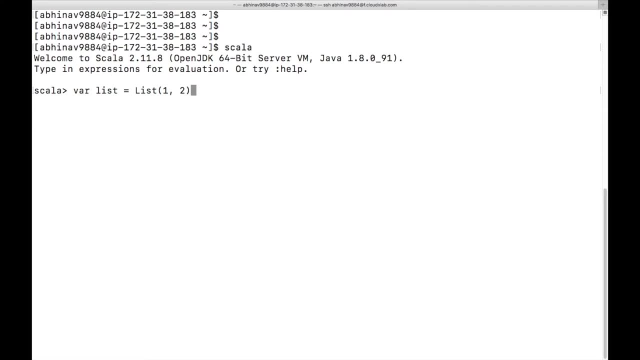 We can use foreach for this kind of scenario, as we do not require an output value To use foreach. higher order function type list: dot foreach bracket. println bracket closed. As you can see, the values 1 and 2 are printed on the screen. 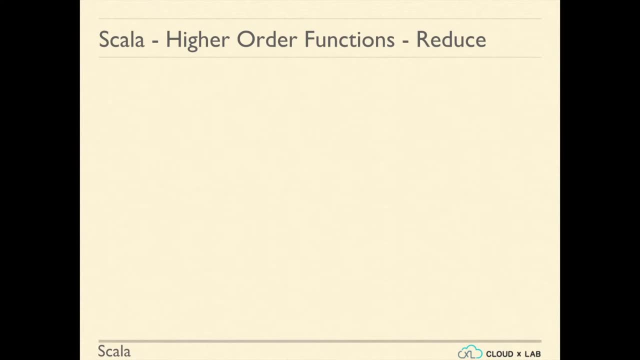 Let us learn higher order function, reduce. Reduce is a very important concept in the MapReduce world. Let us say we have a list and we would like to compute its sum. Let us understand it with an example. We have a list of integers 3,, 7,, 13 and 16..